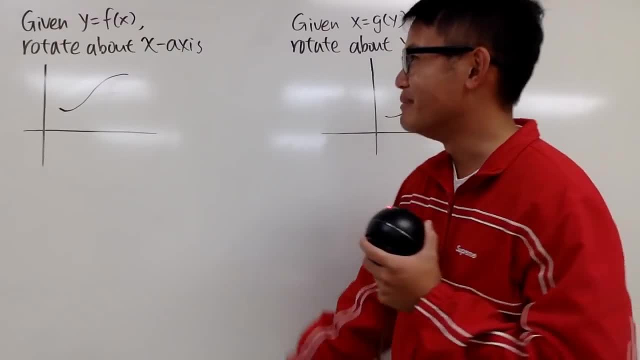 Okay, in this video, let's talk about volume. This is how we are going to do it. Let me show you. Suppose we have a curve right here, and suppose that we are given y is a function of x that describes this curve, and it's similar to the area video that we have. Well, in the area situation, we want to find the area under this curve. So that means you go down from the curve to the x-axis, so you want to find the area of that region. That's the easy situation. You just have to integrate, and you just pretty much do y times dx and all that. Here's the deal though. For this kind of volume situation, we are going to do the following. We are going to take that region, and we are going to rotate that about the x-axis, and that's the easiest situation when you have y as a function of x. Once again, I will take this right here, once again this region, and I'm going to rotate about the x-axis, so the picture is going to look like this. 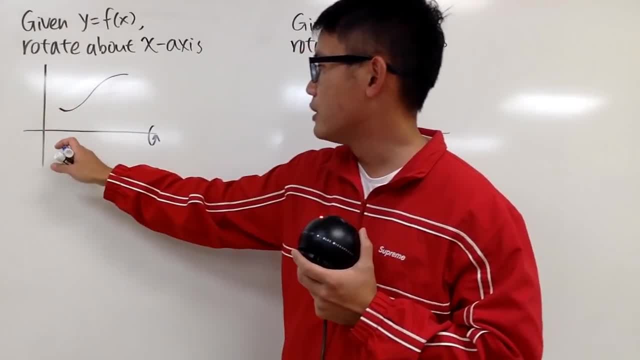 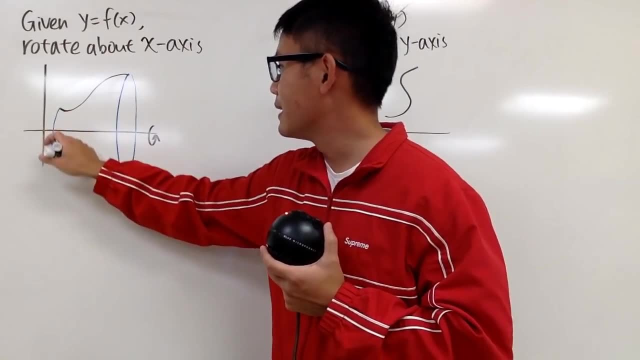 Well, what you can do is you can just kind of mirror the image, and you just kind of practice your drawing skill like this, and you do this and that. That's pretty decent. You can see that's 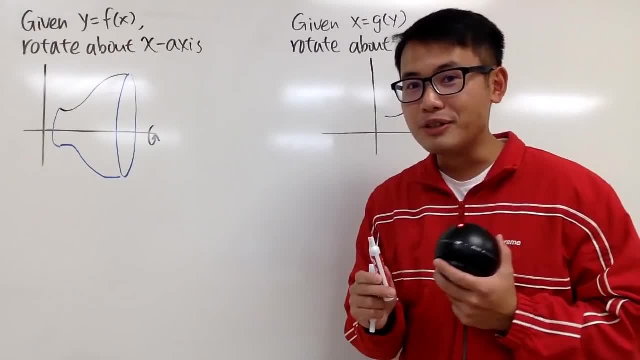 like a 3D picture. So this is an easy situation, and we don't need anything too fancy to do it. 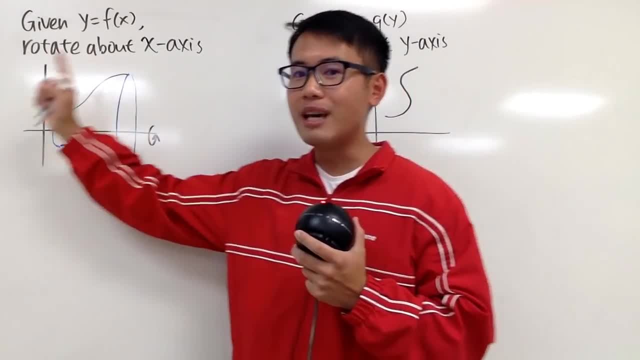 The only hard part is that if you take this region and rotate about the y-axis, that will be the more difficult situation. And the easiest way to take care of that situation is what we have to show 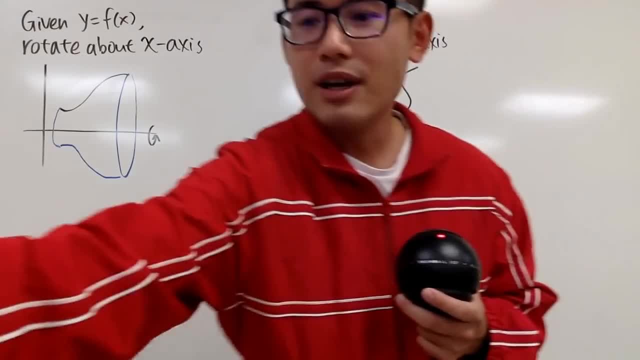 here. But in this video, let's talk about the following. So here I have a bunch of this, which you know, maybe some of you guys haven't seen this for so long, because you know, these 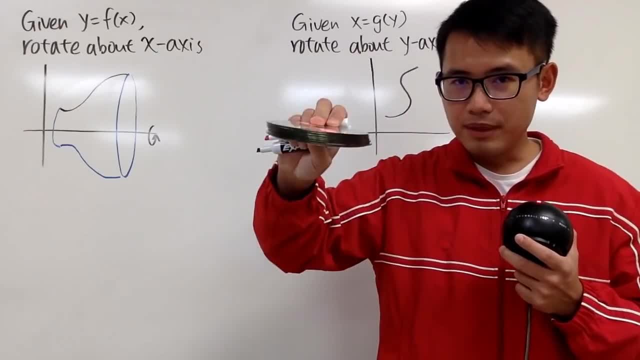 have been outdated, of course. Anyway, describe the shape. If you look at this, these are pretty much cylinders, right? Well, the idea is that I'm going to pretty much 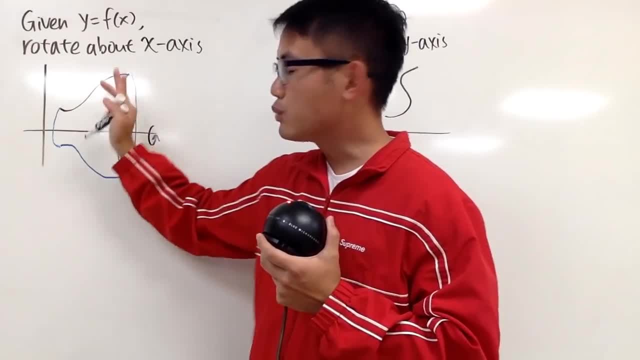 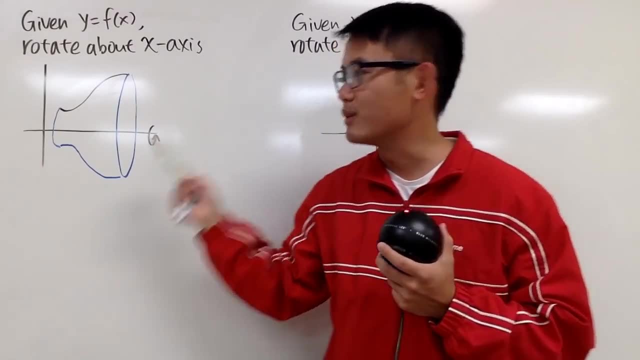 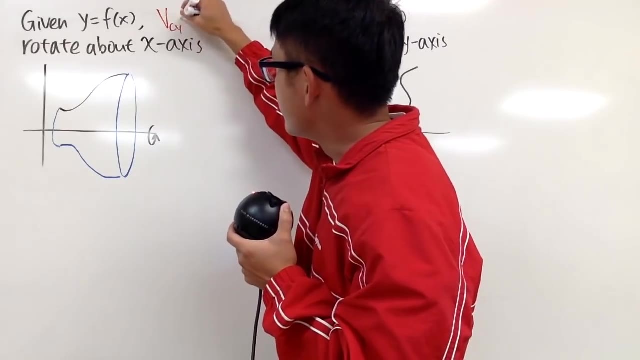 cut this volume, this solid, this way, and each little cut, it's going to be a small cylinder, a CD. That's why this is called the DISC method. And let me also write this down on the side for you guys. Remember that the volume of a cylinder, this right here is just pi r squared, because you 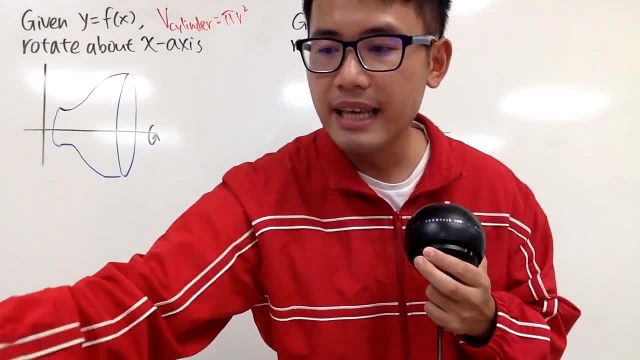 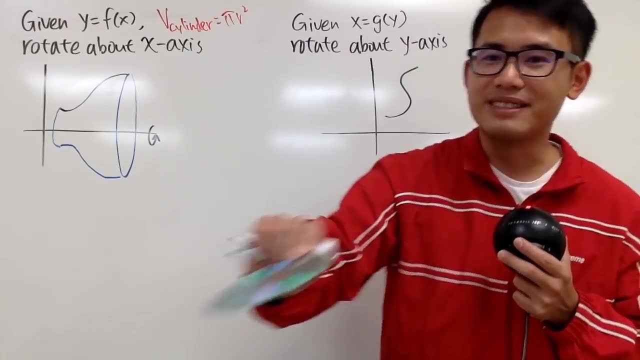 have the area here, and you have to multiply by the height, like how tall this is. But since we're talking about something that's really thin, like a CD, I will not put down the height, I will put down thickness. So I'm going to put down the height, and I'm going to put down the thickness. 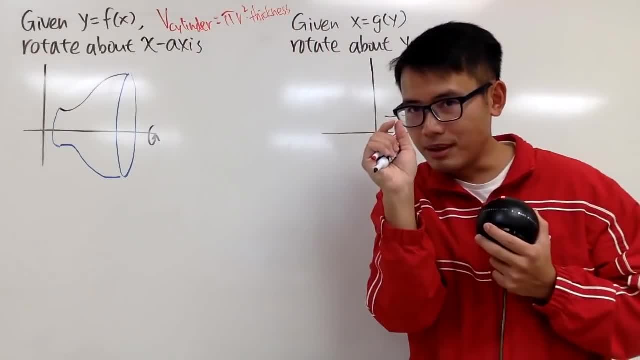 So that should remind you, we're just talking about the little change. 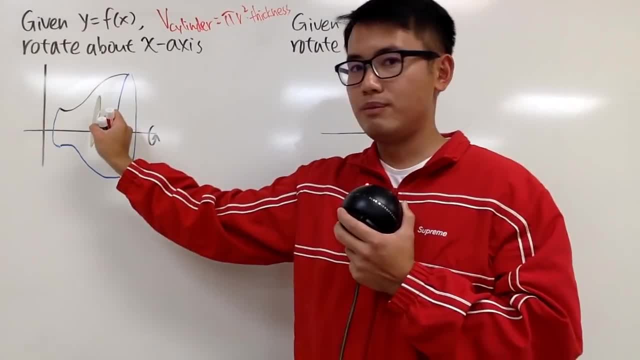 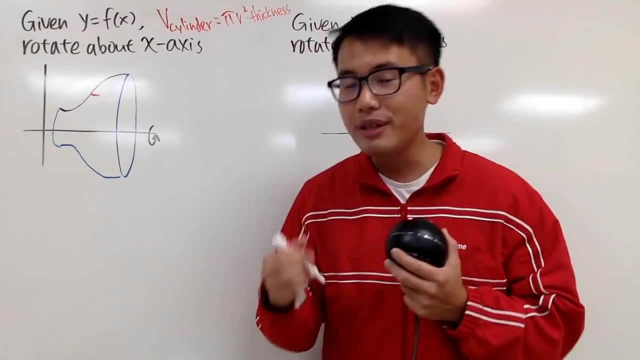 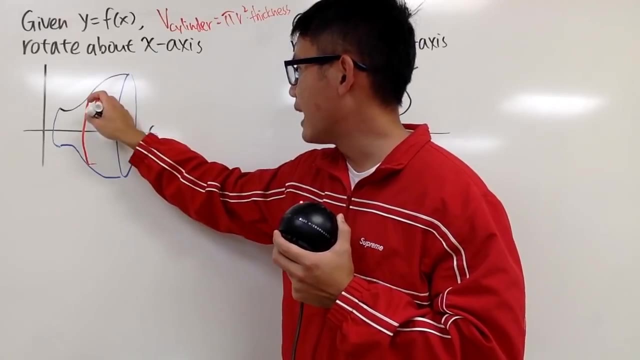 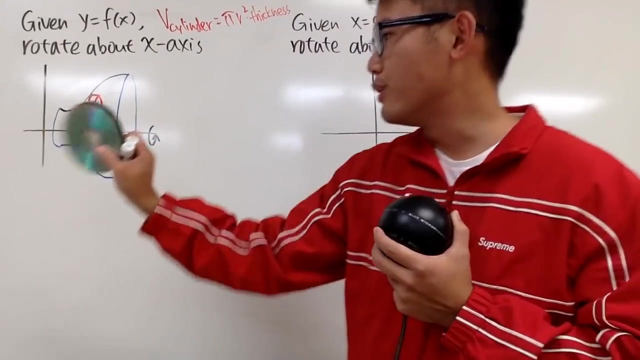 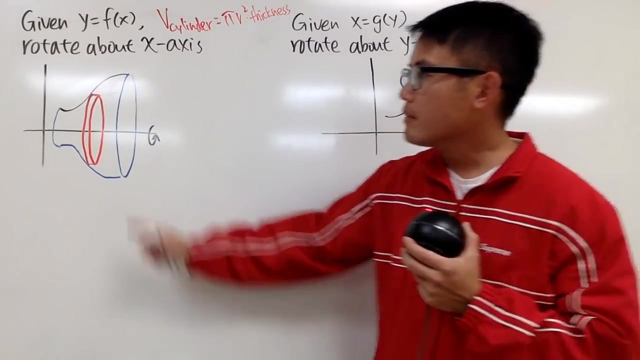 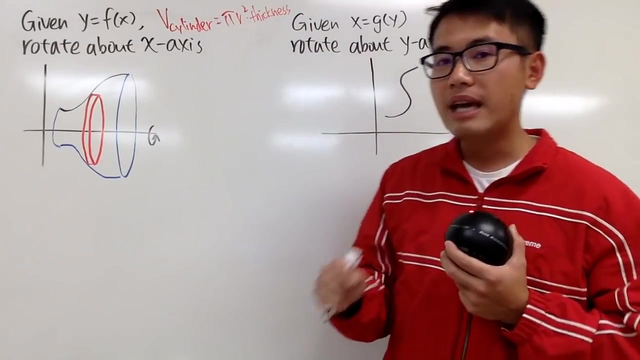 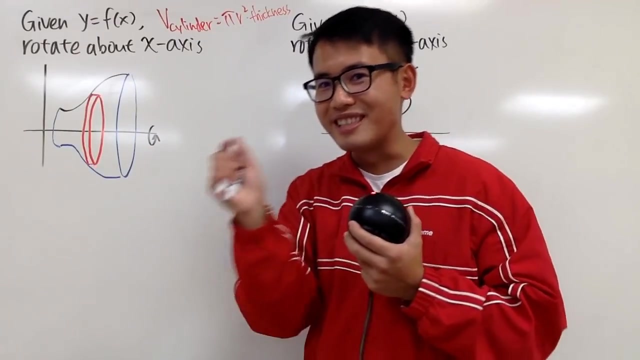 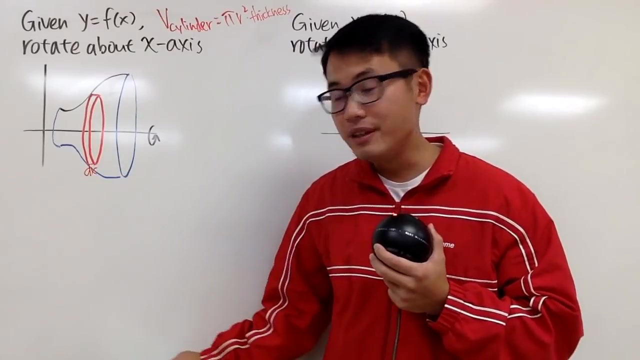 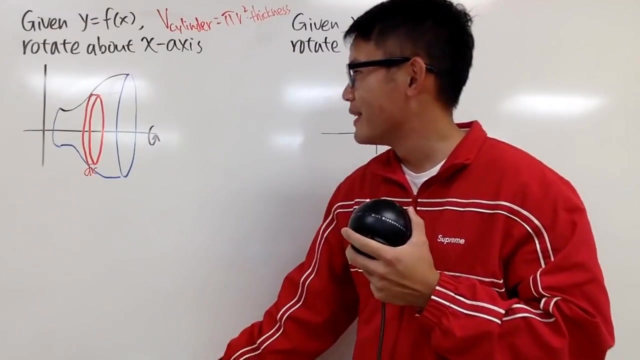 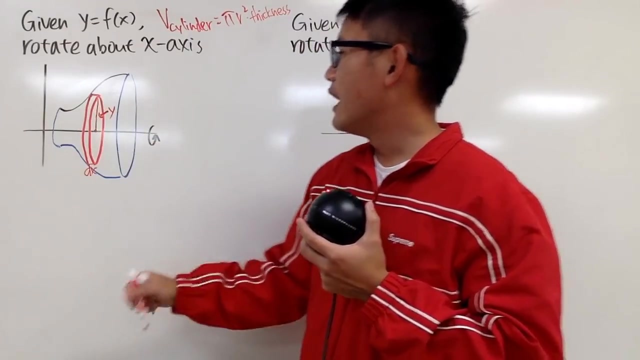 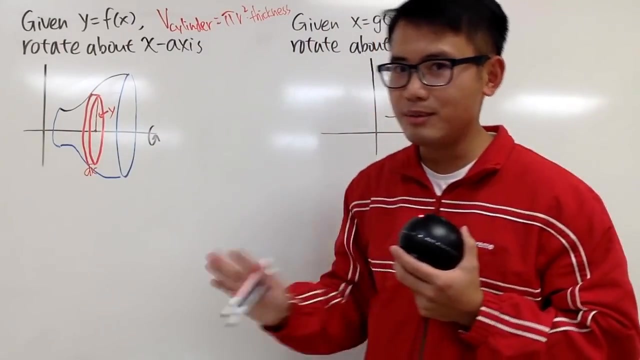 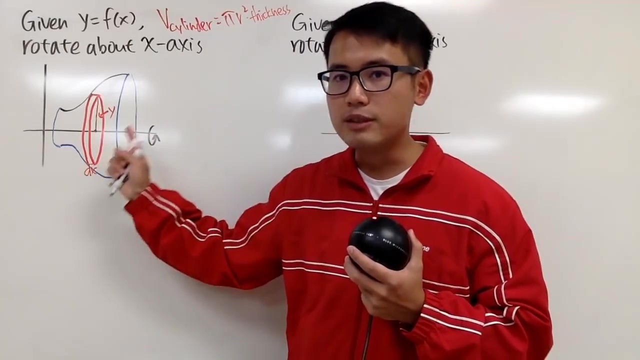 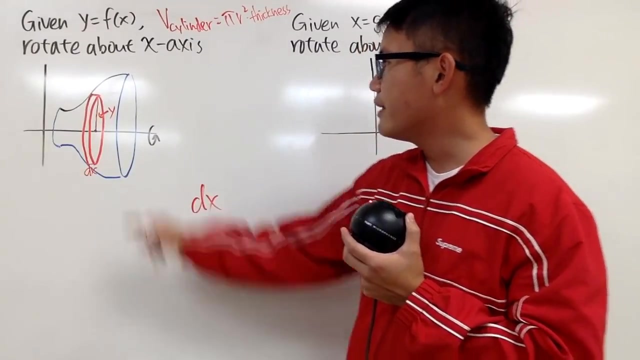 Anyway, the idea is that you put the CD this way, right? So I will draw the little picture here. It's really similar to the area video. We still do this, but this time you are going to draw a disc like that. This red part is meant to be a disc. And the idea is, once again, you're just drawing a bunch of these discs, and each disc, they have different radius. That's the key. Now, I'm going to focus on getting the volume of this red disc. Once again, pi r squared times the thickness, and let's take care of the thickness. If you look at this right here, the thickness is this, which is just a small change in amount in the x values. Therefore, this is just the x. And for the radius, well, as you can see, this is equal to the radius of the disc. And then for the see here is the center, radius means you go from here up, here is the center, the radius means you go from here up, and that's pretty much the y. And you might be wondering, hey, I didn't really touch it, but you know this is supposed to be really thin, so the y is pretty much right here. Once again, it's seriously similar to the area video. So that's pretty much it. Now let's write the volume of this red disk. We will have the thickness is dx, so let me just put that down right here, and then the radius is the y, so we will have 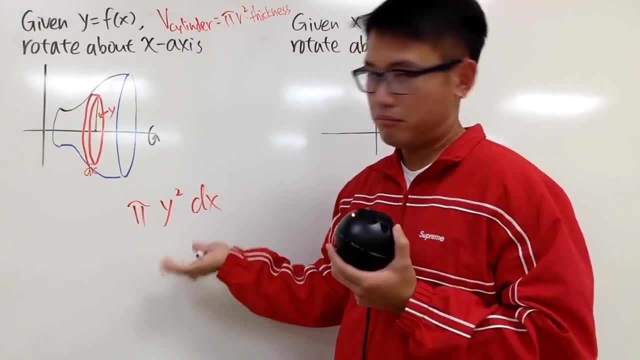 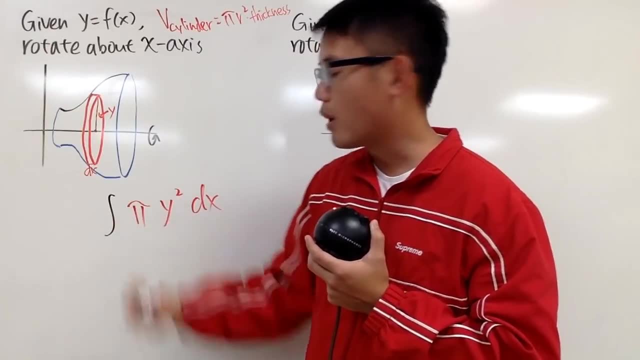 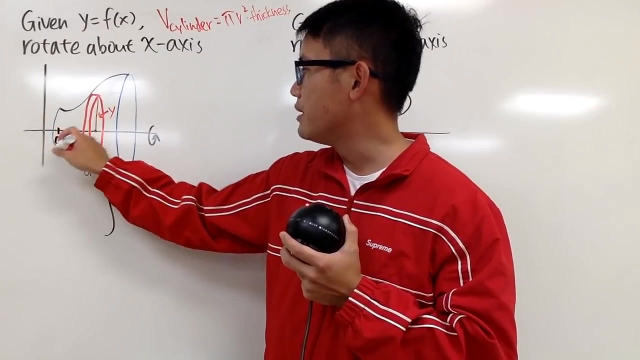 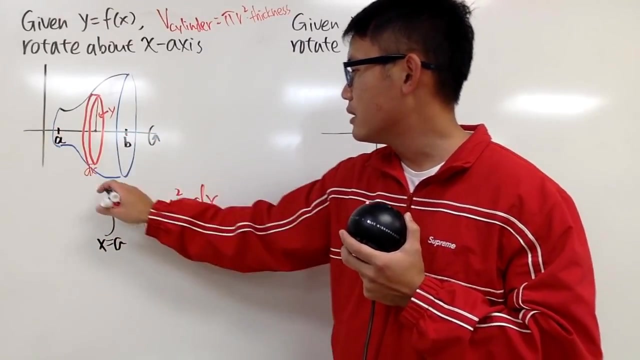 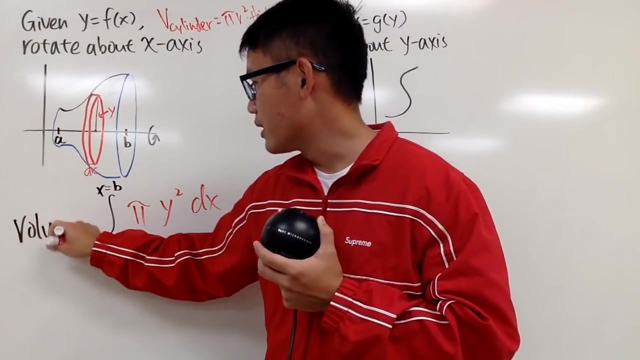 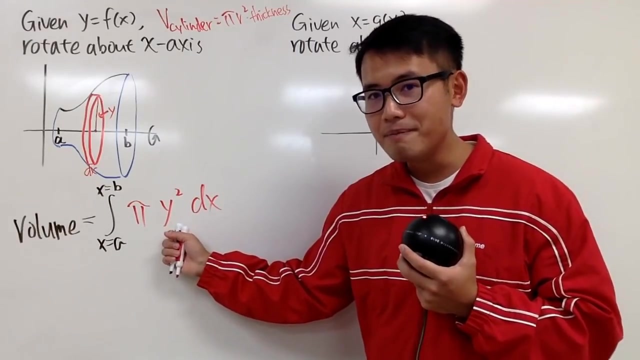 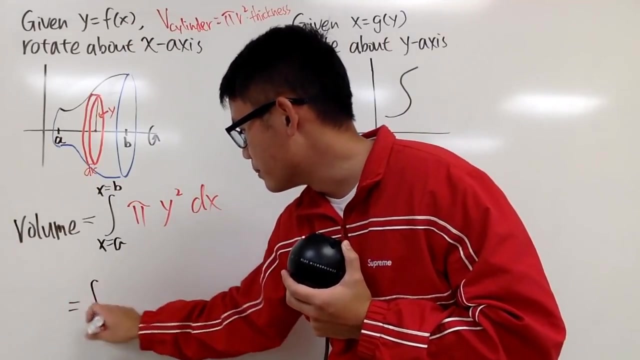 to just square the y, and then pi is just a pi, that's pretty much it. Well, well, we have to add up all of this disk, so we will have to just do the integral, and we are in the x world, so we have to go back to the picture and see maybe the beginning. The beginning x value is a, so I will say, hey, we have to go from x is equal to a up to the ending x value that says b, where x1, x2 doesn't matter. That's pretty much it. So if you do this, you can get the volume of this solid. And of course, if you would like to know why it's not invited in the x world, so just put the function in here, and that's pretty much all. So in the end, we see that the volume is just a to b. 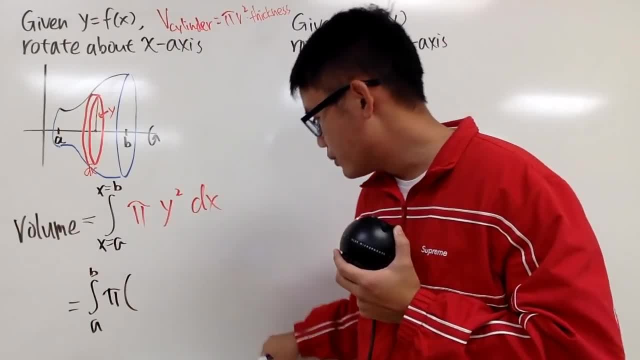 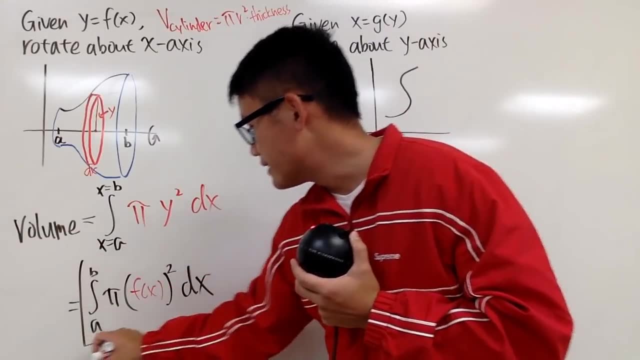 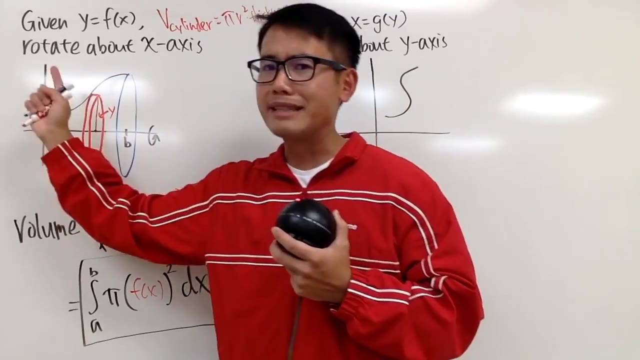 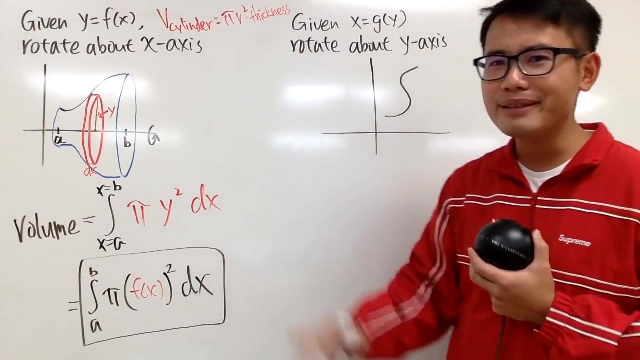 Pi times the function, which is f of x, let me just put this down in gray like this, f of x, square that, dx. And as I said, this is the easy situation. The harder part is that you take this region, you rotate about the y-axis, or maybe rotate about y is equal to negative 1, or you take that, rotate about x is equal to 17, things like that. This is the easy way. This is the easy case. All right. 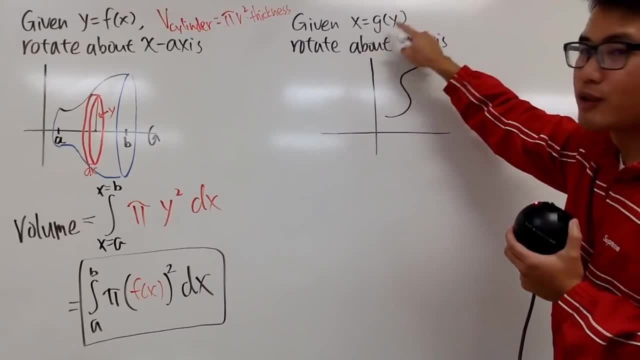 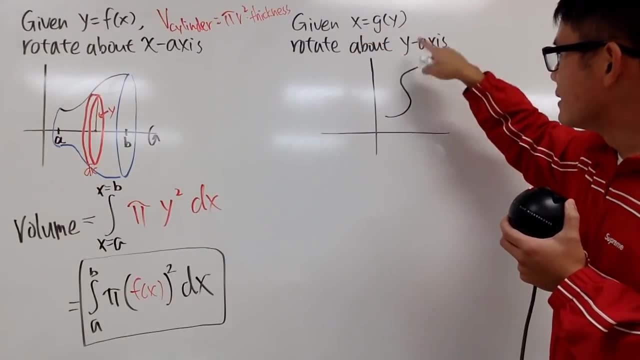 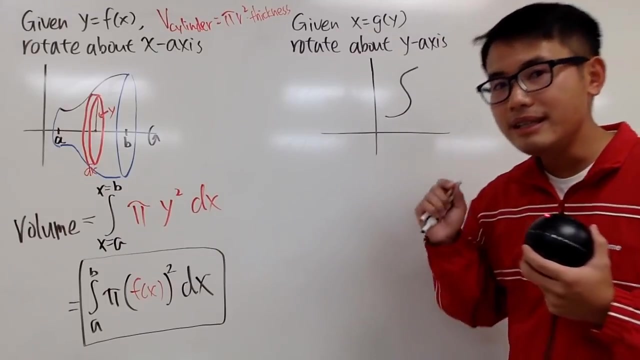 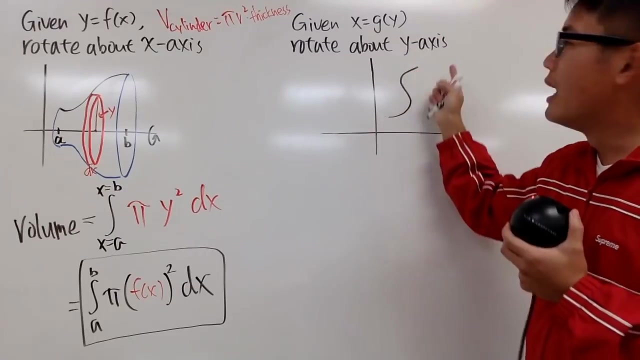 On the other hand, we might also have x being a function of y. And you see, if you look at it this way, OK, that's like the graph of x as a function of y. This is not a graph of y as a function of x, because it doesn't pass the vertical line test. Anyway, when you have this situation, the easy way to do it is we want to rotate this region, suppose you go from here up to here, that region, about the y-axis. So you just go ahead and do this to remind yourself. 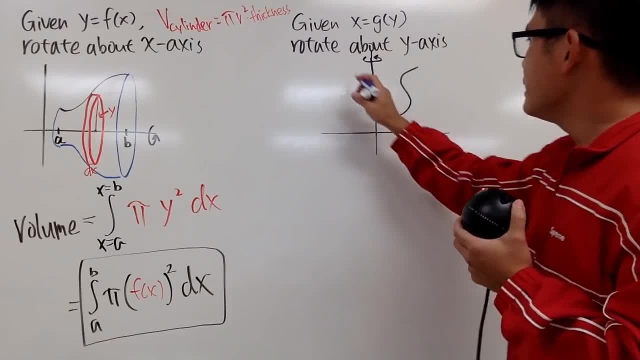 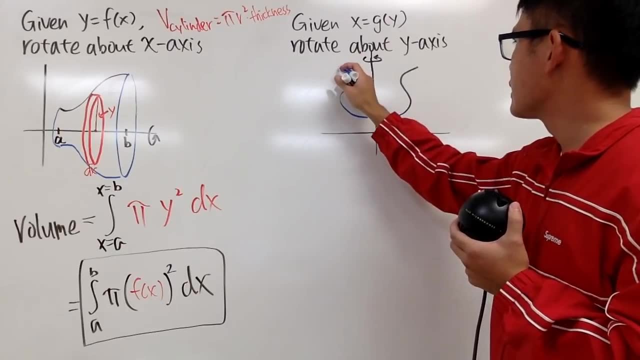 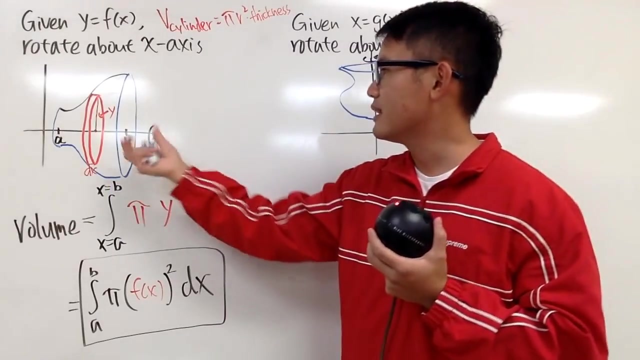 We are rotating about the y-axis. And to draw the picture, you pretty much, once again, just mirror image. You'll see, like this. And then on the top, do this. On the bottom, do that. So this is like this. And this is, I don't know, like this, the other way. I don't know. Yeah, you can leave a comment down below and let me know what do you think 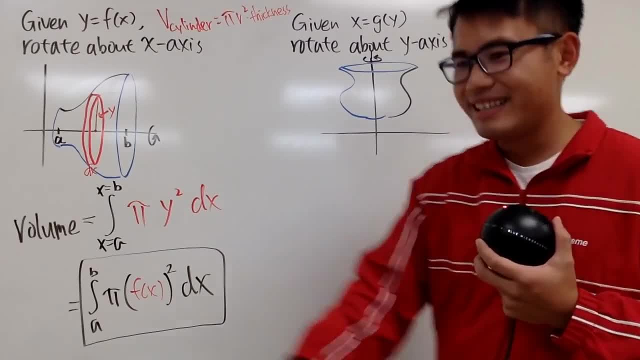 about this kind of picture. This time, we are going to put a bunch of CDs horizontally this way, isn't it? 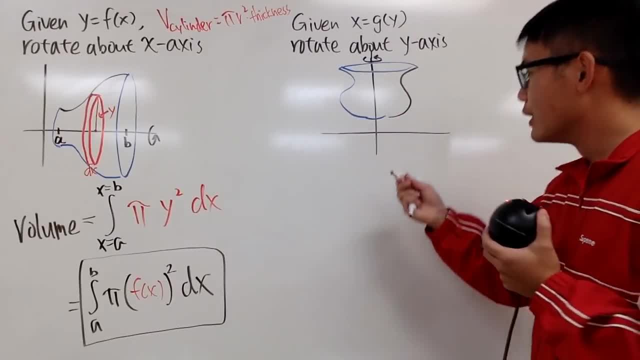 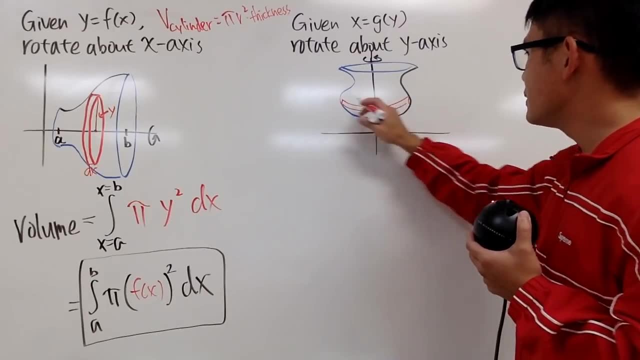 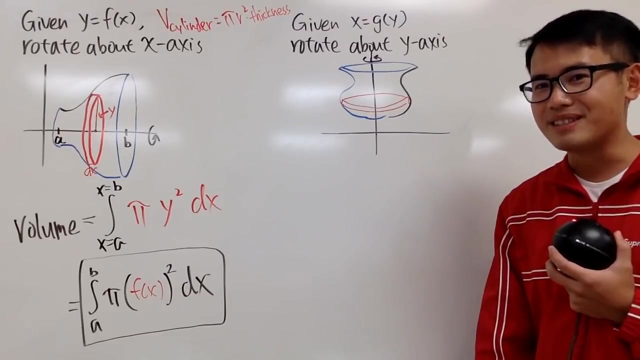 So we are going to draw the disk this way. Don't just focus on the formulas. Seriously, focus on how we approach solving the questions, because later on, when you guys do some work on some physics questions, this is the technique that we use, right? Anyway, here's the deal. 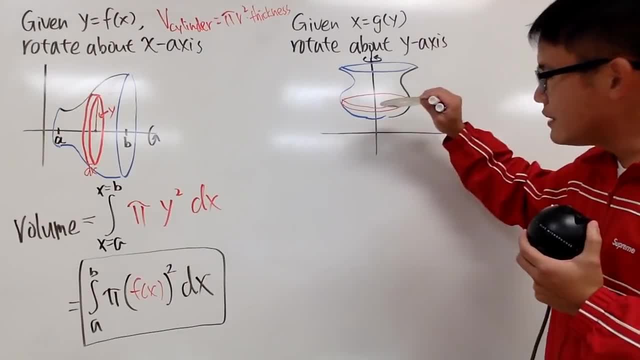 You draw this red disk. It's a horizontal slice. Now you have one CD. You want to find the volume of this CD.